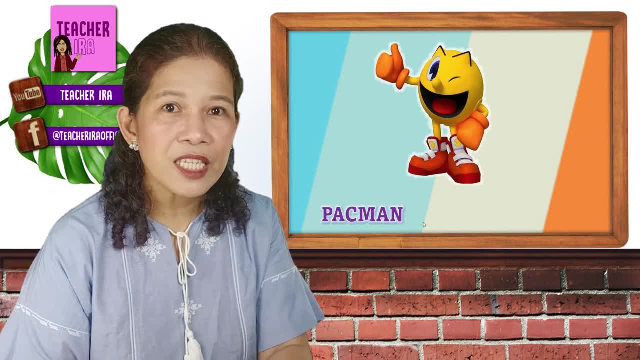 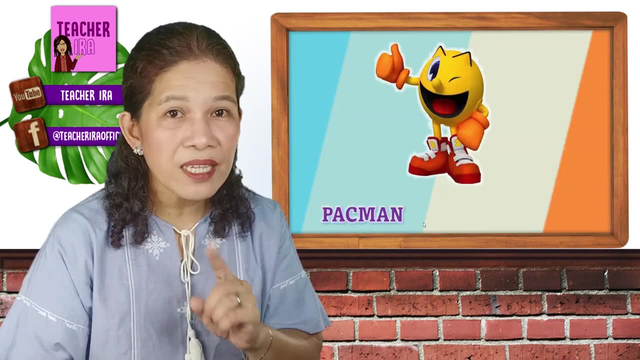 Hmm, what does Pac-Man do? Yes, Pac-Man would love to play this game. Pac-Man would love to eat more, more, more, more more. That's why, for you to be able to write the symbol properly, you think about Pac-Man. 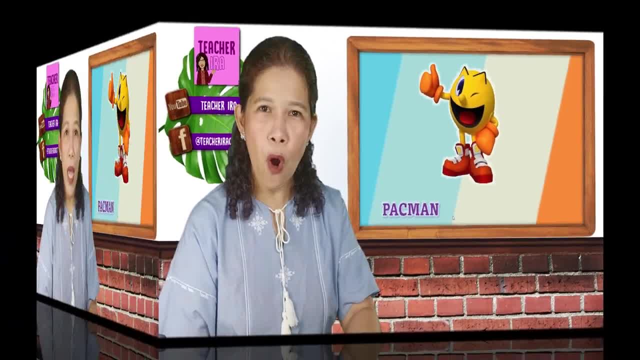 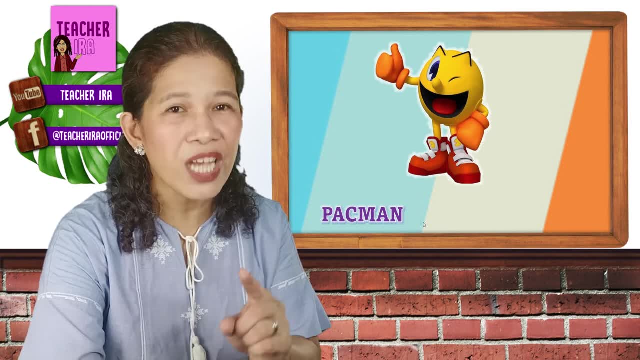 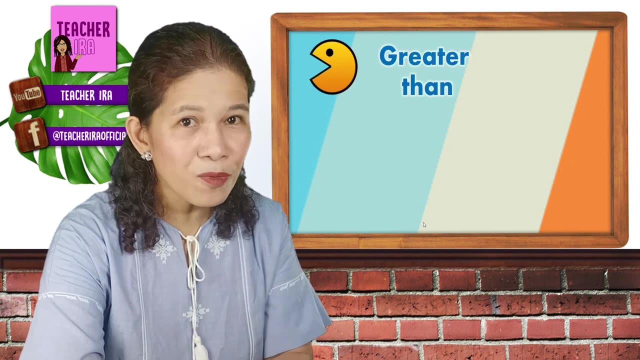 Always remember that Pac-Man would love to eat more. And now we will make use of his mouth. Of course, we will not draw the whole Pac-Man character, but just his mouth. Okay, now, when a symbol greater than we will use the mouth of Pac-Man this way. 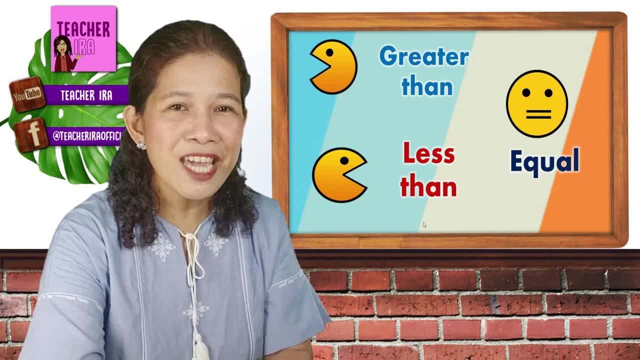 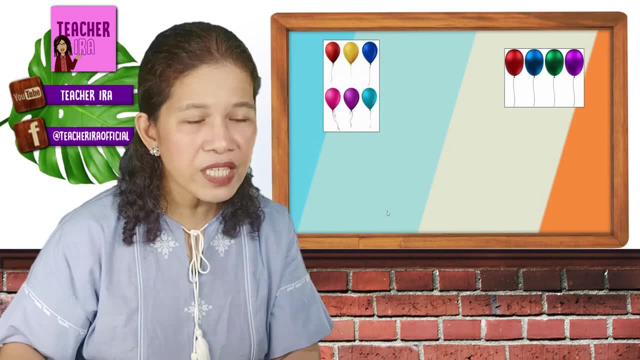 And then less than would be this way, And equal- Equal would be this way. Okay, let us have an example. I have here two sets of balloons. On the first set, we have here one, two, three, four, five, six balloons. 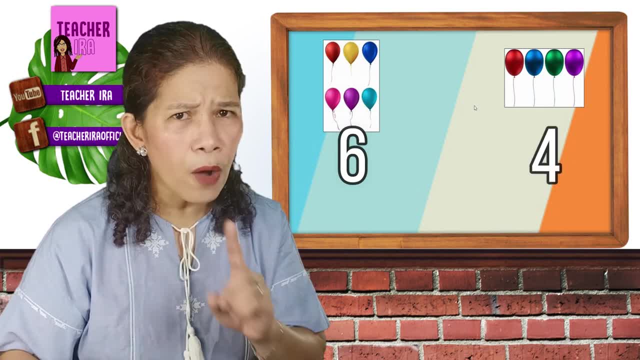 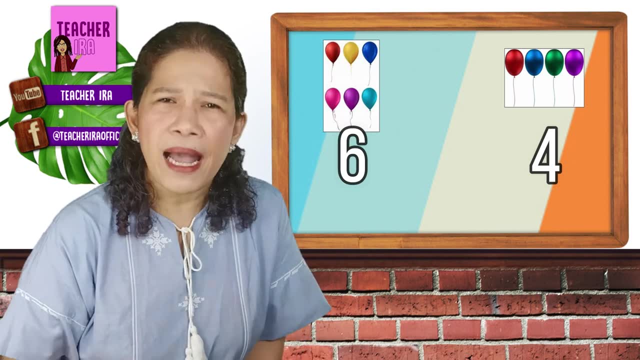 And on the other set we got four balloons. Now which set has more? Yes, the set with six. Now, what do you think will Pac-Man eat? The one with six or the one with four? Remember, he loves more. 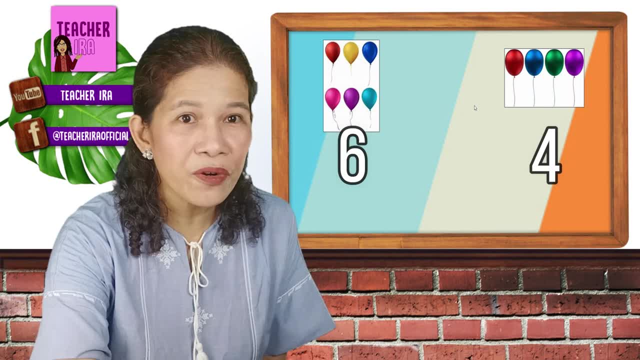 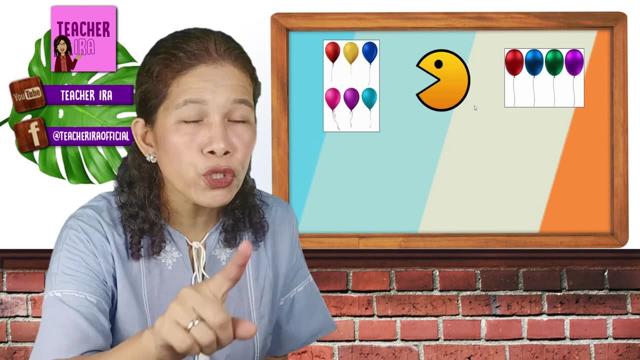 You are correct. You are definitely correct. Look, Pac-Man will eat the set with more. That's why you have to open his mouth. You draw the symbol that has the mouth facing to the set with more. Are you getting it now? 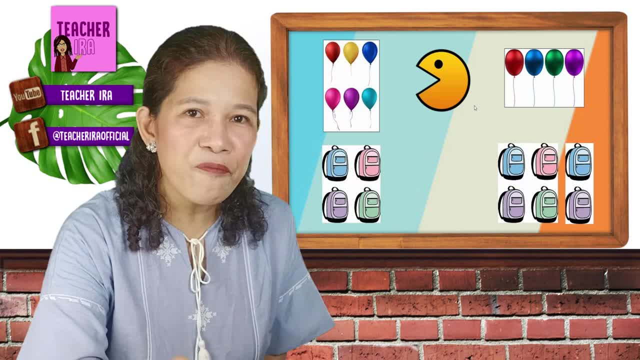 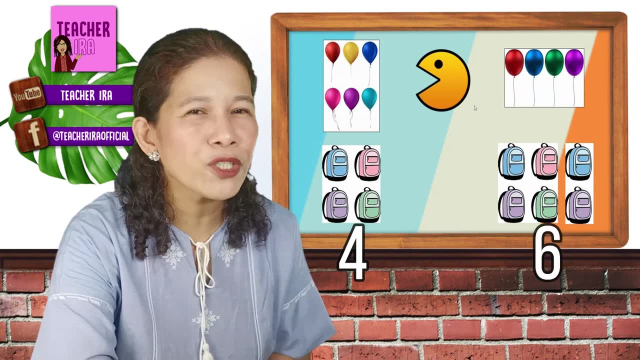 Okay, let me have another example. Okay, I have here a set of bags. Okay, the first set has four and the other set got six. Now, what do you think will Pac-Man eat? The one with four or the one with four? 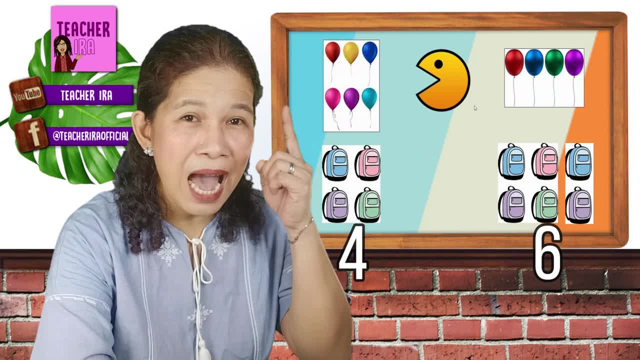 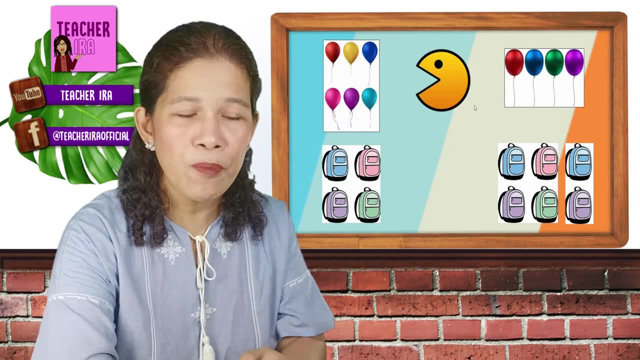 Or the one with six, Of course, because I've told you that he loves more. You think about that. Okay, his mouth would be opened to the set with more. Now, when you have this one, you would say four is less than six. 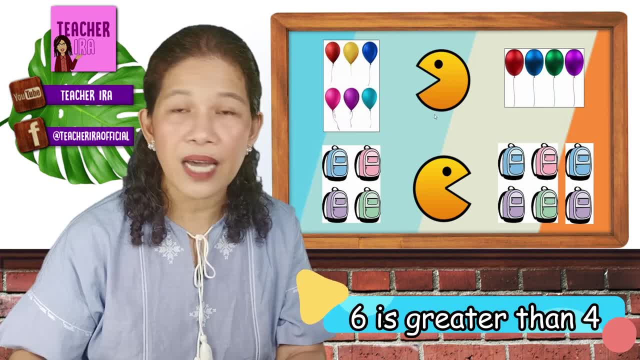 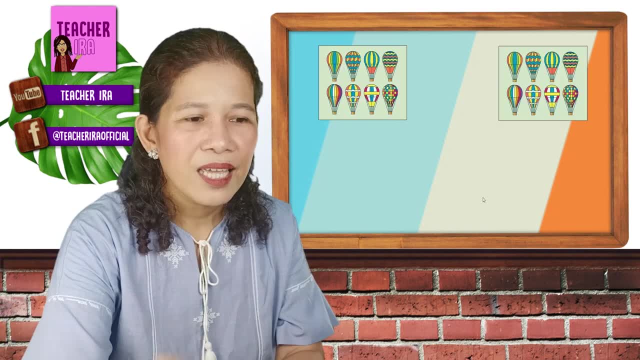 And the other one up here would say: six is greater than four. That's how you understand: the greater than and the less than. Now let's have some more examples here. Okay, here, Whoa, We got two sets, Two sets here of hot air balloons. 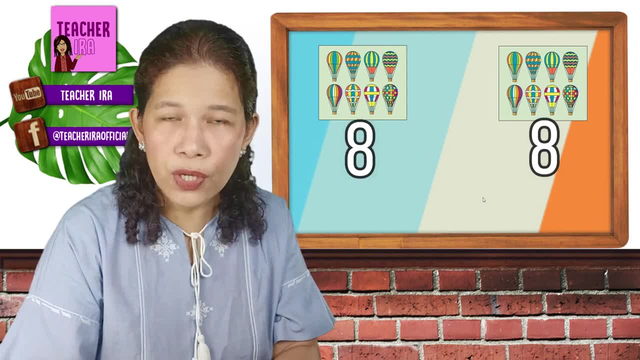 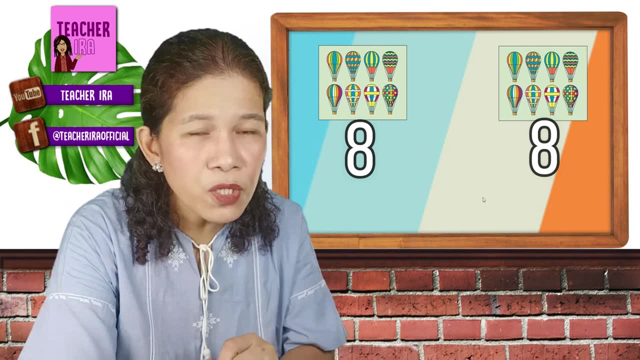 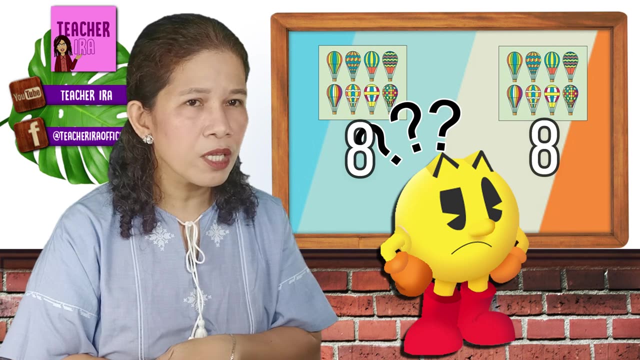 The first set got eight, and the second set got eight too. Now we have the same number of elements here. So, hmm, when it comes to that point, Pac-Man will think: should I eat the one here on this side, this side, or on this side? 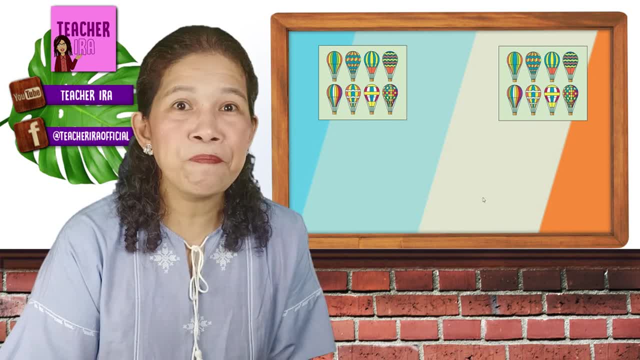 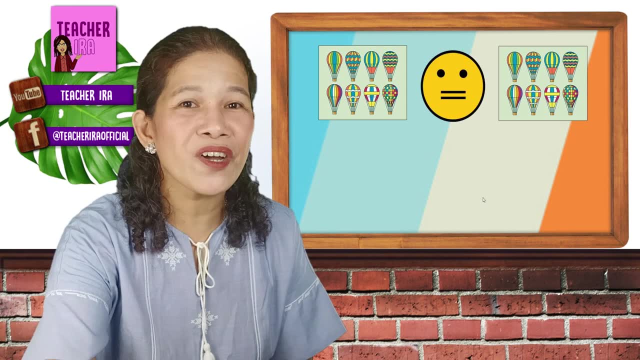 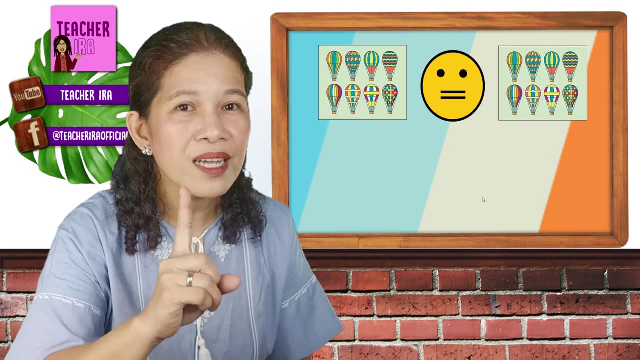 And then suddenly his mouth would say hmm, because he could not decide what to eat. Now look at the mouth of Pac-Man, So it's gonna be equal. His mouth would be like that because he could not decide as to what set is he going to eat. 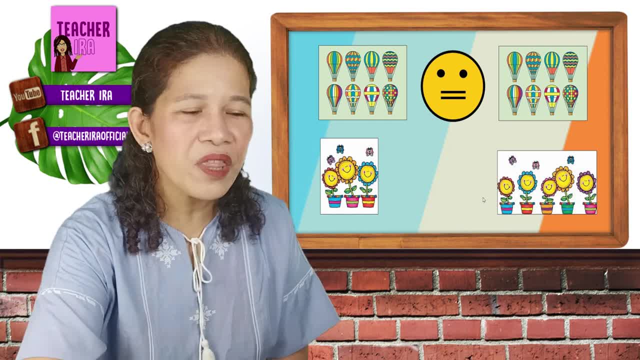 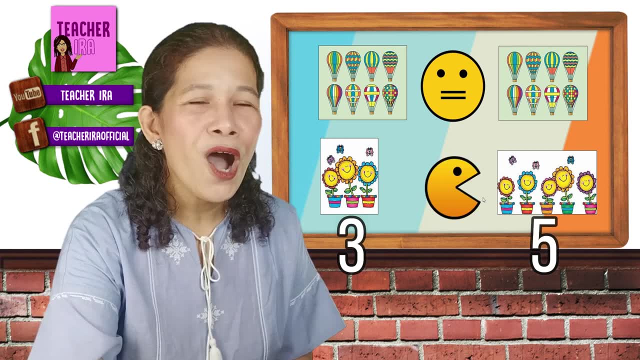 Hmm, you're getting it now right. Okay, now, how about with this set of three and five? Is it greater than, less than or equal? Of course it's gonna be. three is less than five, Pac-Man will eat it. 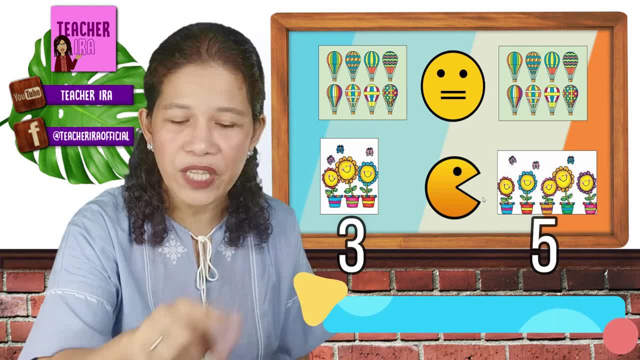 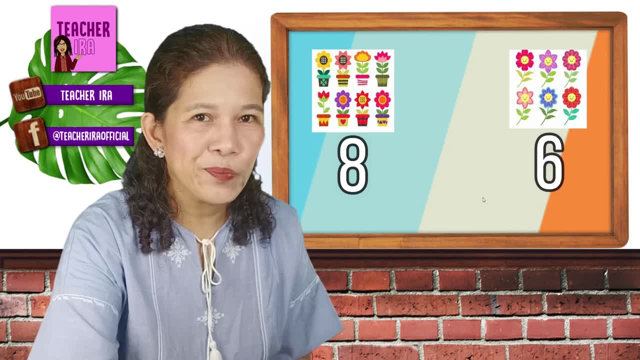 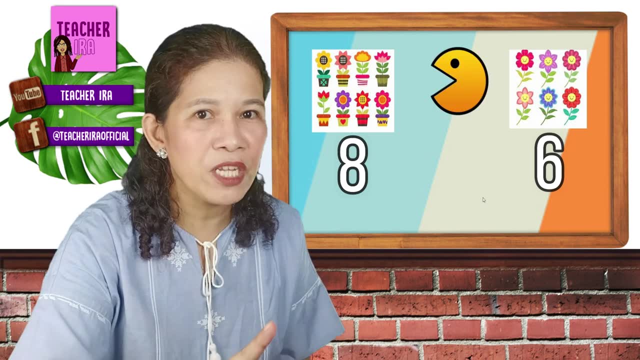 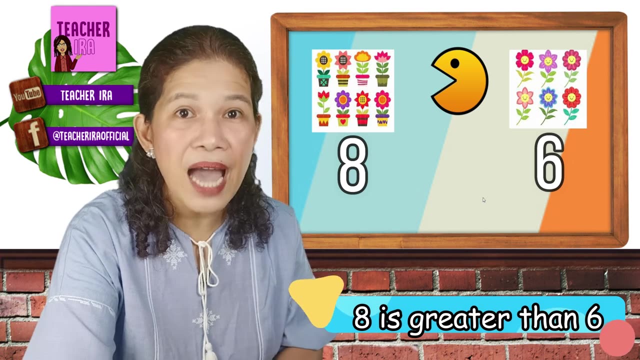 Okay, eight and six. Hmm, greater than or less than or equal? Yes, of course, because Pac-Man will open his mouth there. So now, that symbol is greater than Eight, is greater than six. Next, four and four. 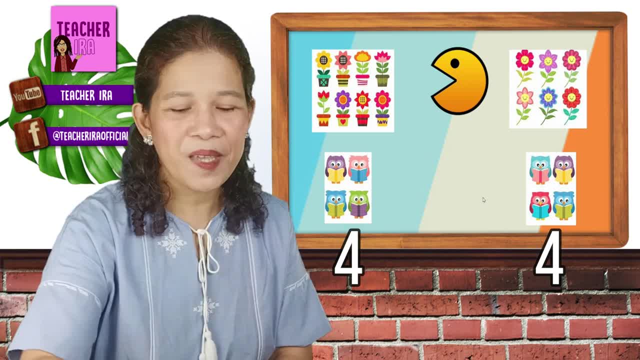 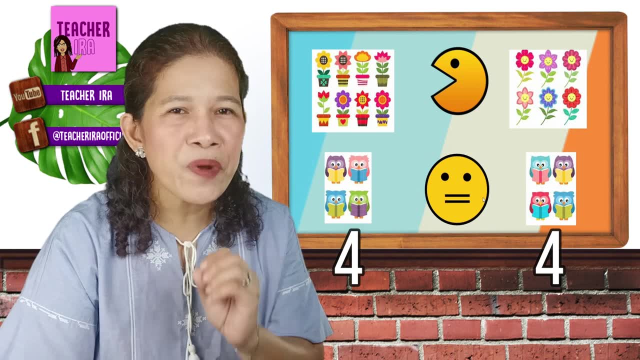 Hmm, his mouth will say hmm, hmm, hmm, hmm. Okay, so that's going to be equal again. Very good, Now are you getting it. Always remember that you will open that mouth to the set with more elements. 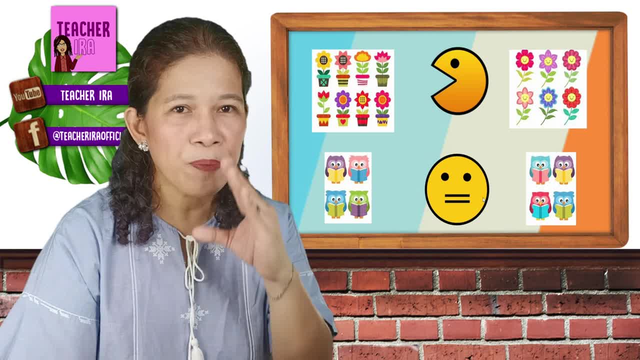 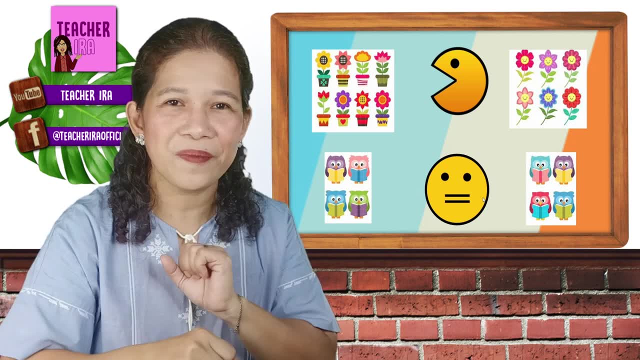 And whenever it faces on that direction, that will be called greater than. When it is facing this direction, it would say less than. When it's like this, it's equal. Now let us try. Can you tell me if it's going to be greater than, less than or equal? 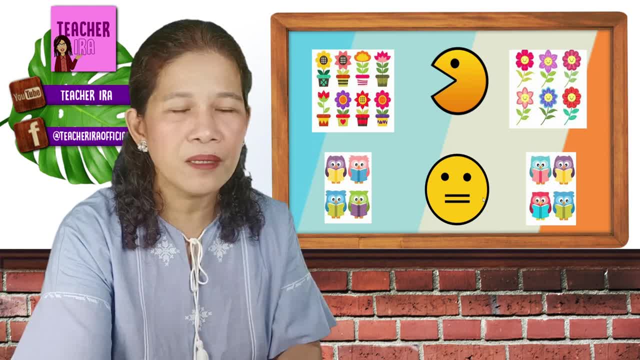 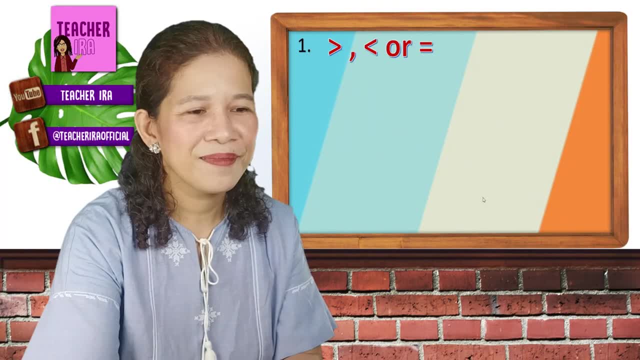 You may have your own paper there, or your whiteboard and a pen, And try to write your own answer. Remember the mouth of Pac-Man kids. Let us try Number one, four and four, Just like what we had a while ago. 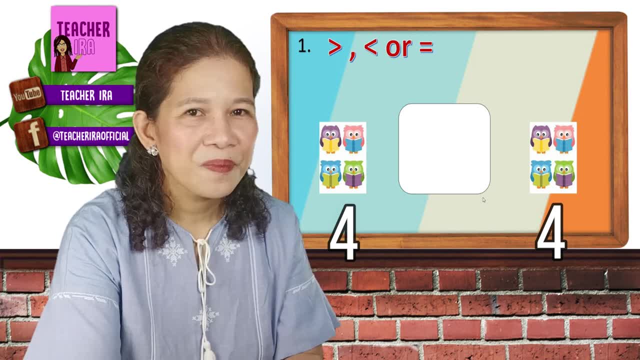 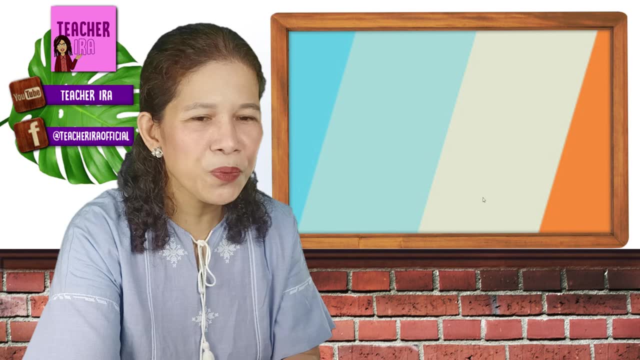 Is it greater than, less than or equal? Yes, it's equal, Correct, You have a star for that, Of course. Now number two: Greater than, less than or equal. Eight and six, Of course, you know that for sure. 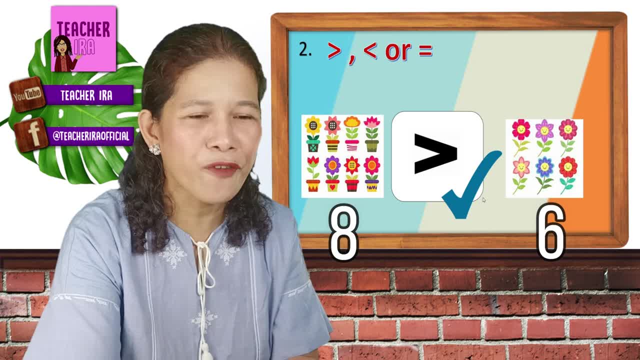 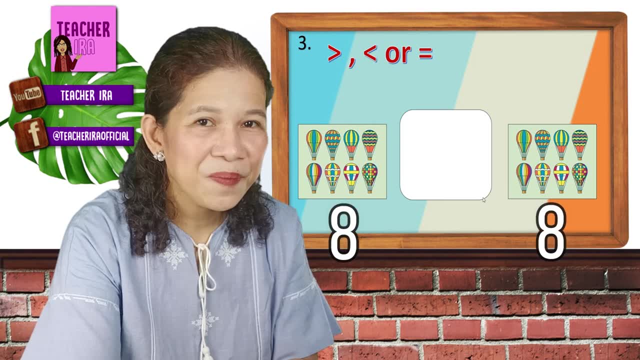 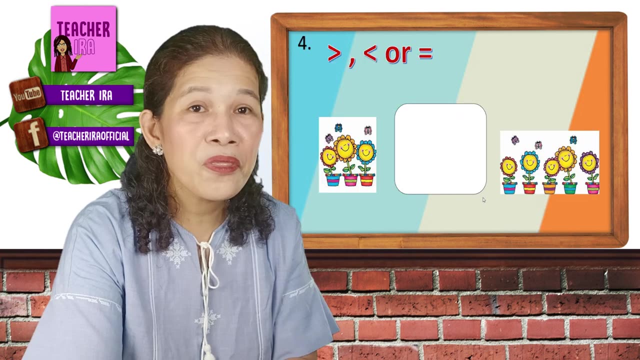 That's greater than Another check for you kids And a star And number three, Eight and eight, That's equal Check, check, check And a star. Very good, Number four, Three and five. We had it in the example. 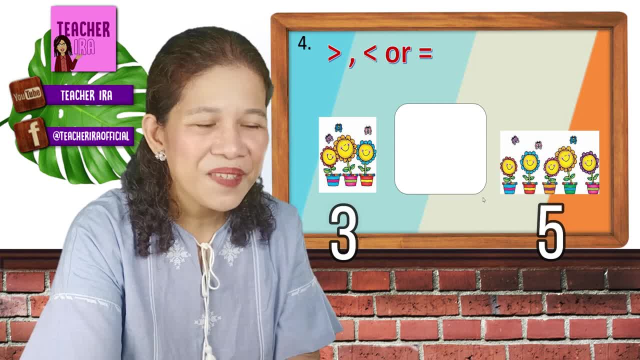 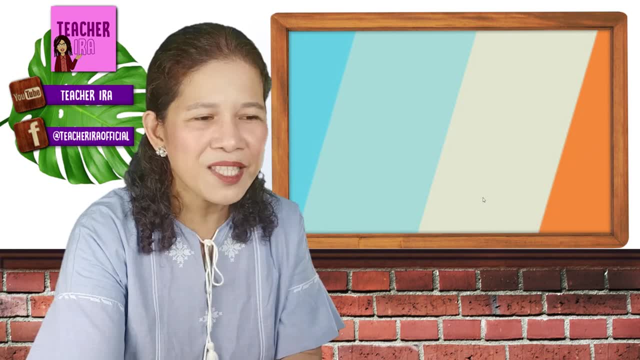 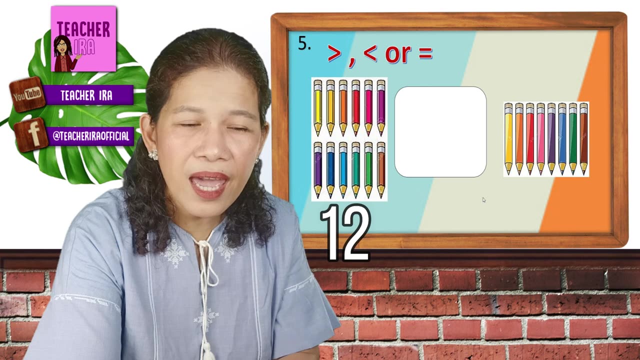 A while ago. Let me see if you can still remember. Yes, that's less than Correct. correct, correct And a star for you. Last, number One: two, three, four, five, six, seven, eight, nine, ten, eleven, twelve and eight. 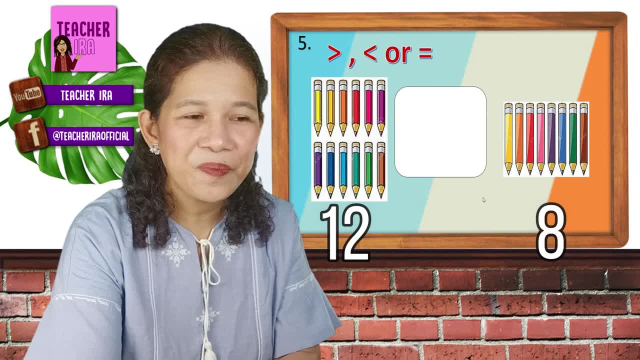 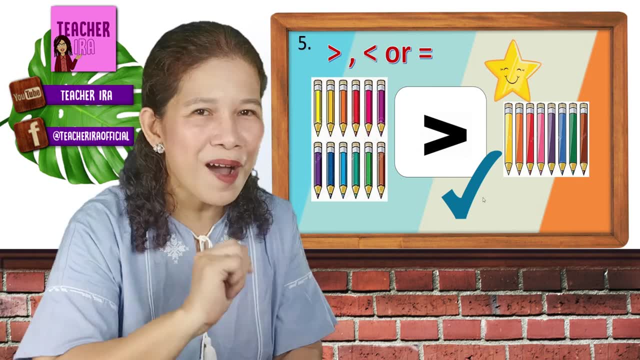 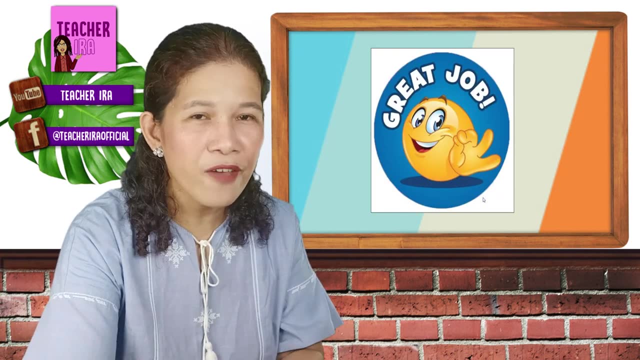 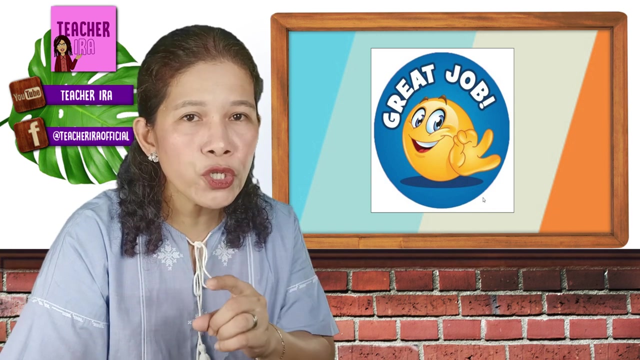 Twelve and eight Greater than, less than or equal. It's greater than. Very good, Check, check and star. Wow. You did a great job if you were able to get five and up Children In comparing the sets with greater than, less than and equal. what you need to do is observe the sets, count and find out which has more and which has less. 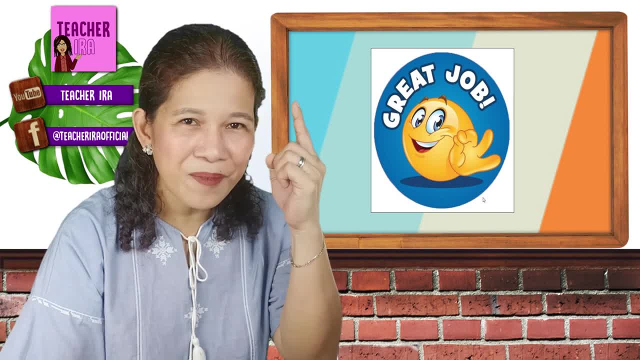 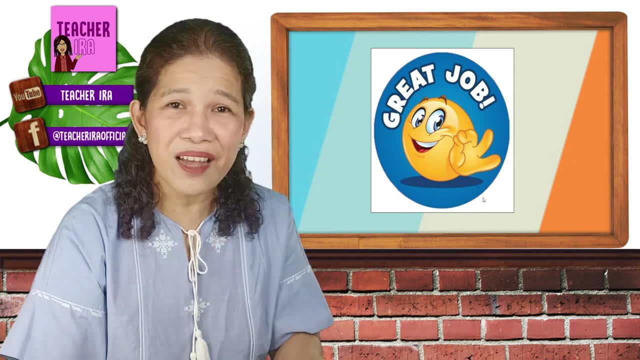 And in writing the symbol, you think about Pac-Man, You think about his mouth And always see to it that his mouth is being opened to the set Because he loves to eat more. Because he loves to eat more, And you will never go wrong. 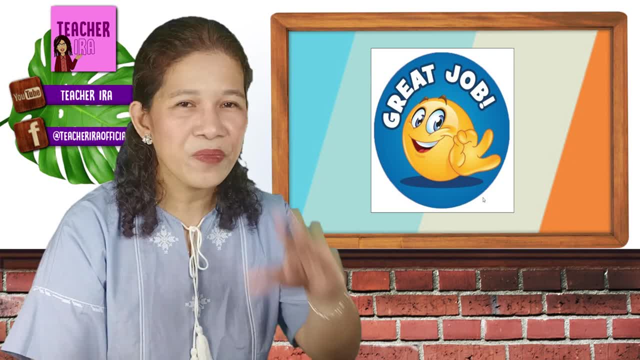 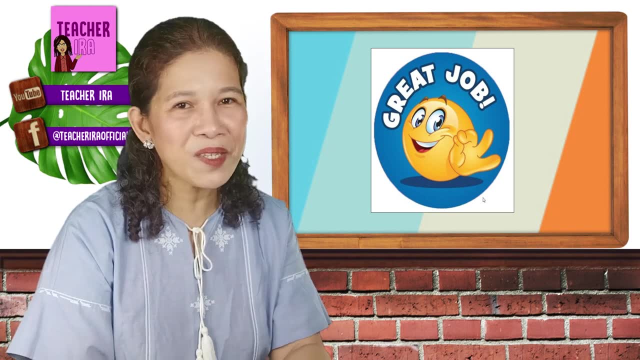 So, one more time, let's name these symbols. You say greater than, less than and equal. I hope that you had learned something today. God bless you. now, kids, Bye, Thank you, Bye, Bye, Bye, Bye. 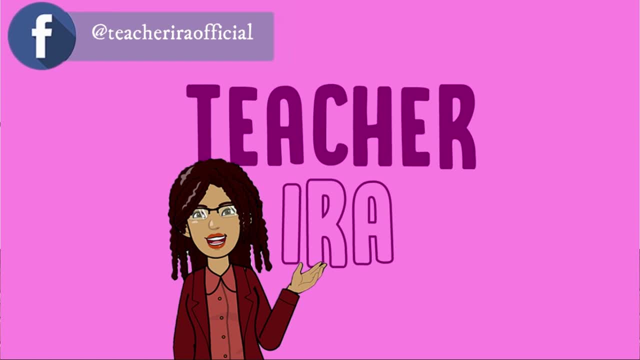 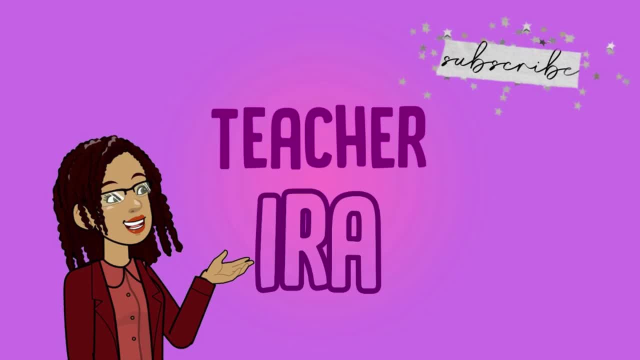